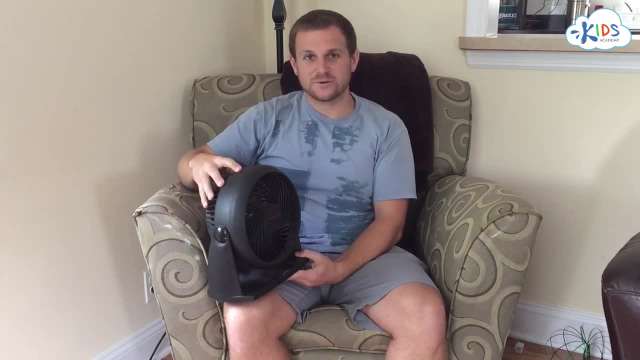 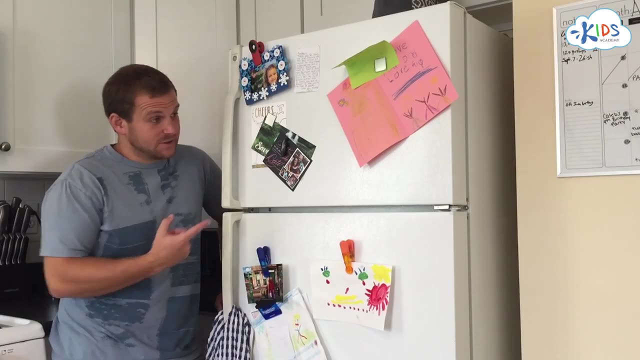 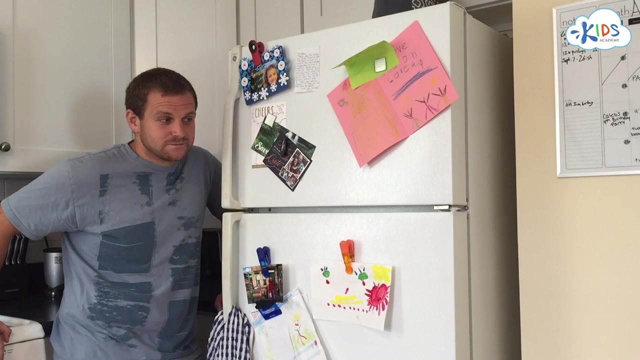 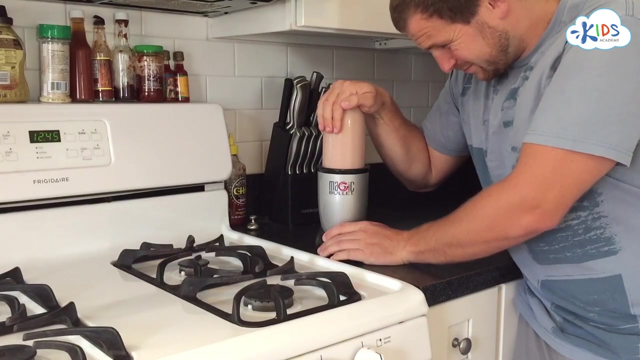 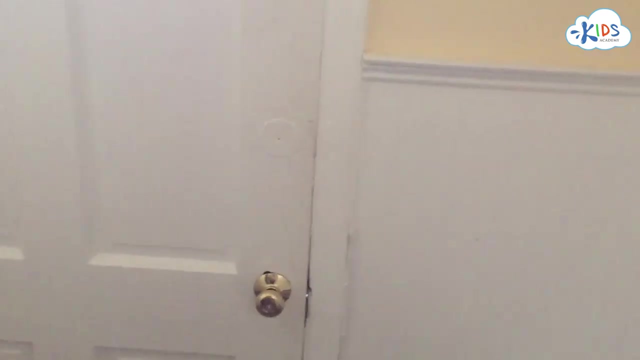 Now that the fan is using energy, we can hear it making sound. We can find sources of sound around the house, Like this refrigerator. If you listen, you can hear it humming. Some sounds are loud, Some sounds are really quiet. Sources of sound are everywhere In our house. 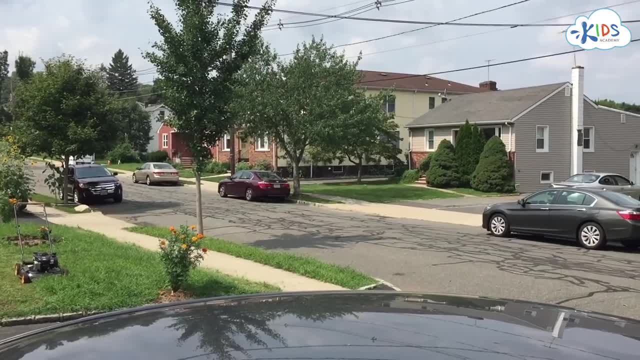 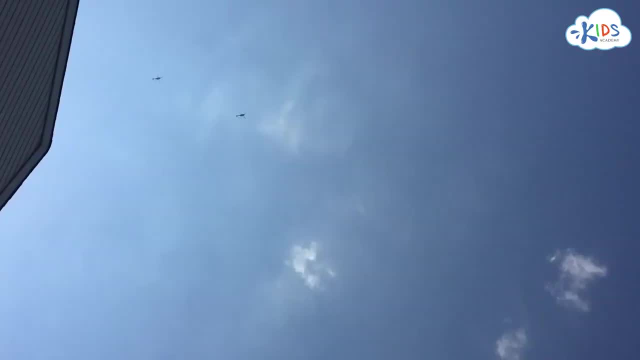 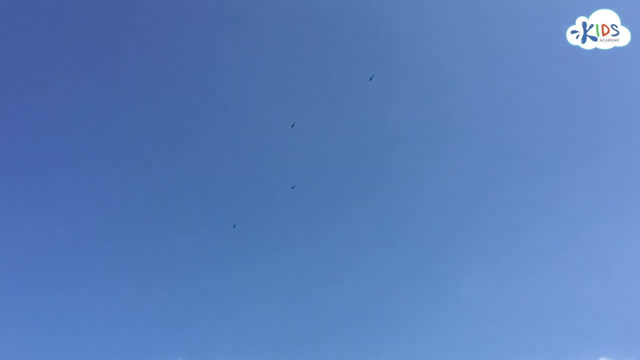 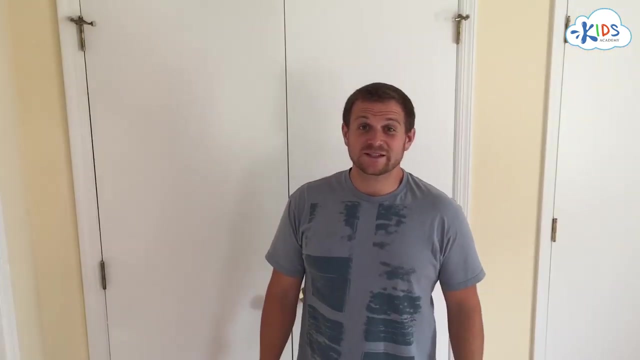 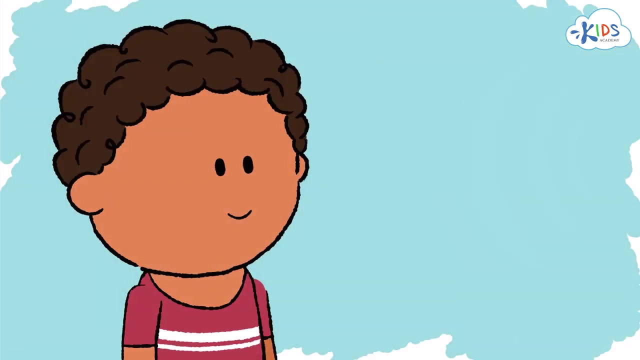 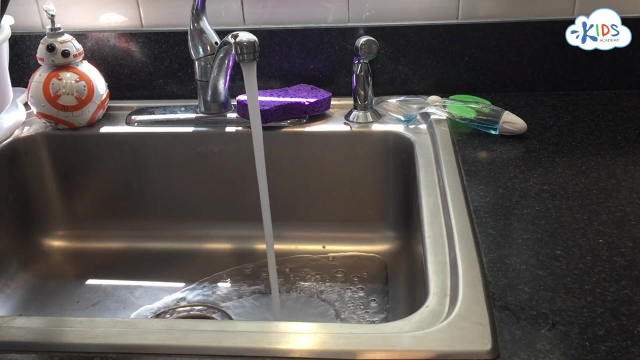 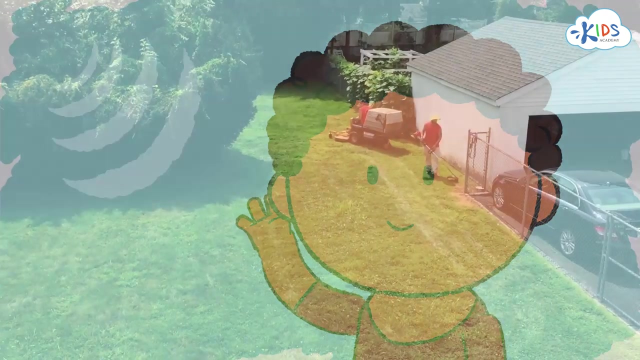 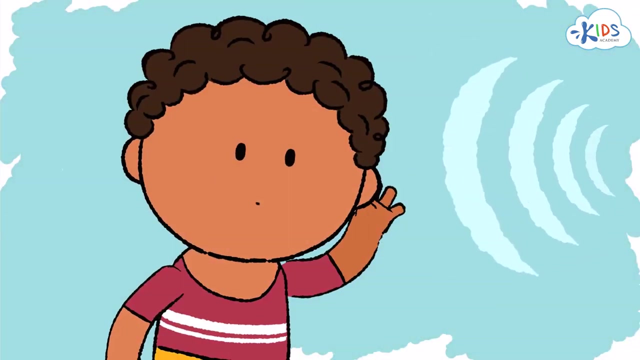 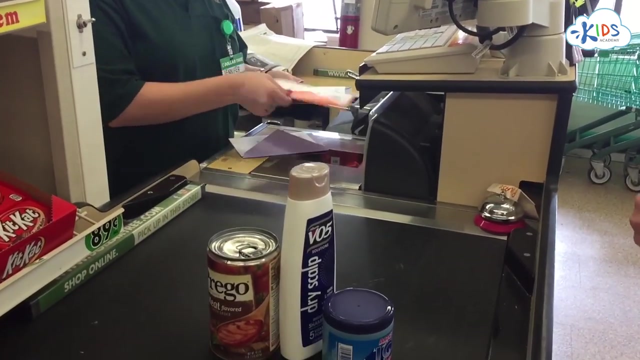 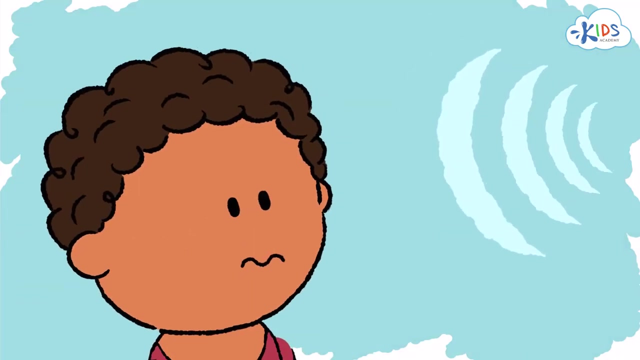 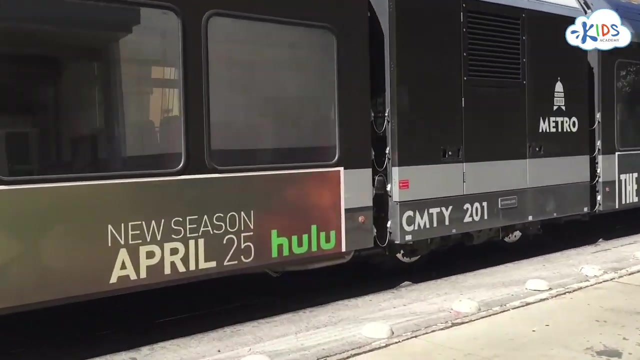 In the streets Around town And even in the sky, Dude-. Now let's see if you can identify these common sounds from around the house and the neighborhood. So, Paulie, what are some of the things that we've learned today? 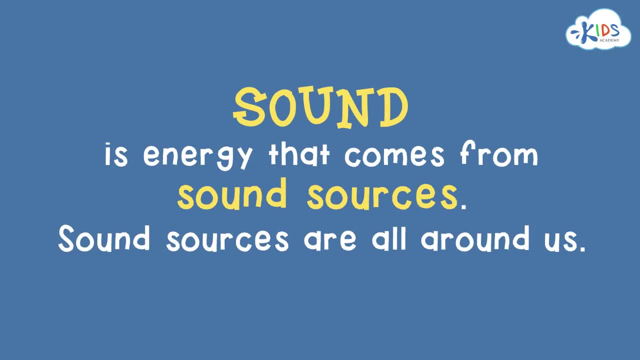 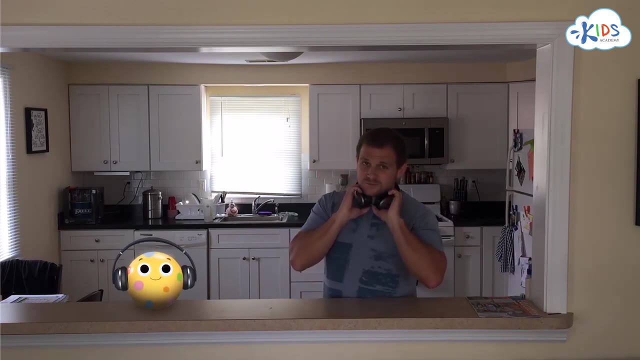 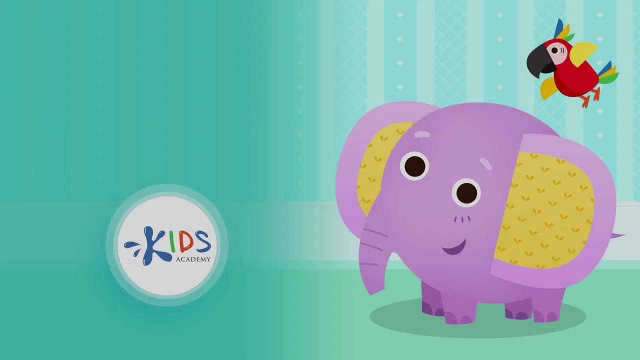 I learned that sound is energy and it comes from sound sources. Sound sources are all around us all the time. That's right, Good job. Now, if you'll excuse us, me and Paulie got some tunes to listen to.